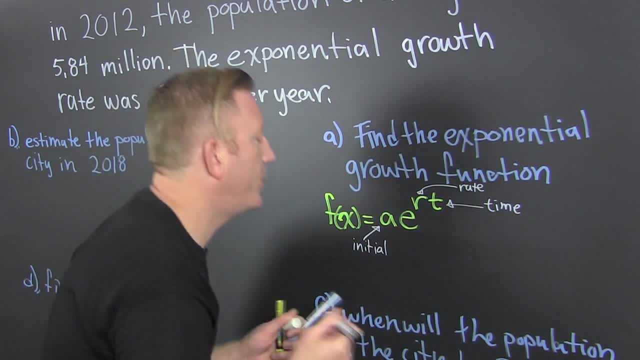 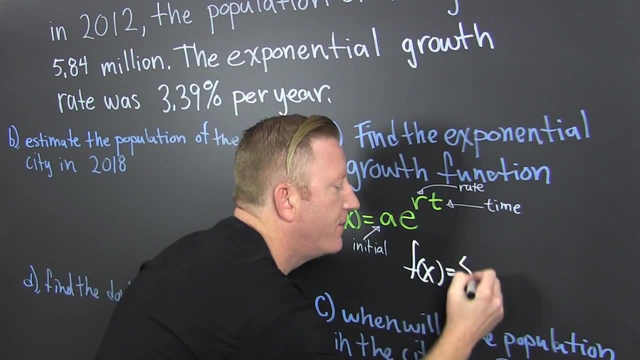 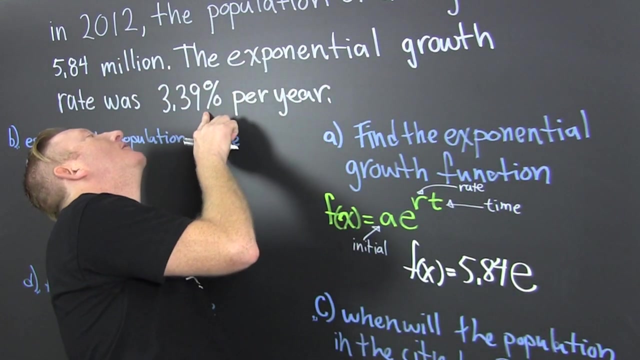 usually in years. Here we find here that our f of x, what was our initial population, Looked like. it was 5.84 million And then it's e to the r. Now r growth rate was 3.39%. How do you write that as a decimal? Move it to. 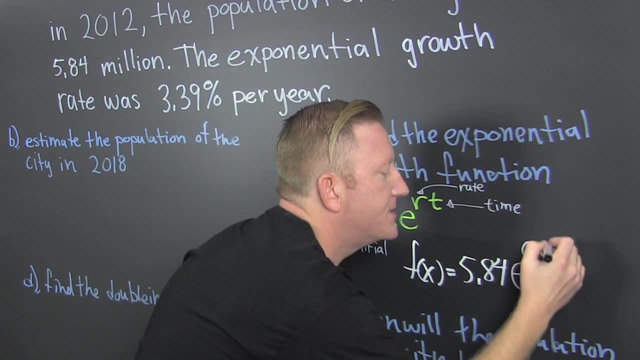 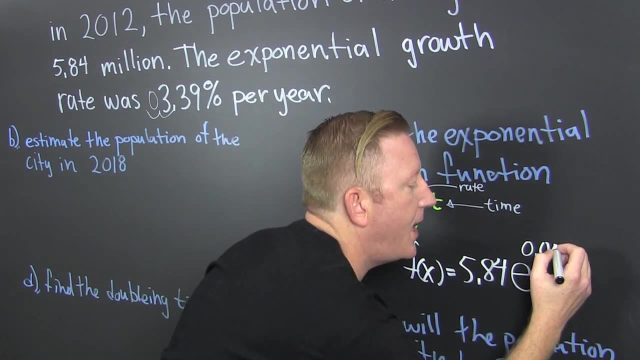 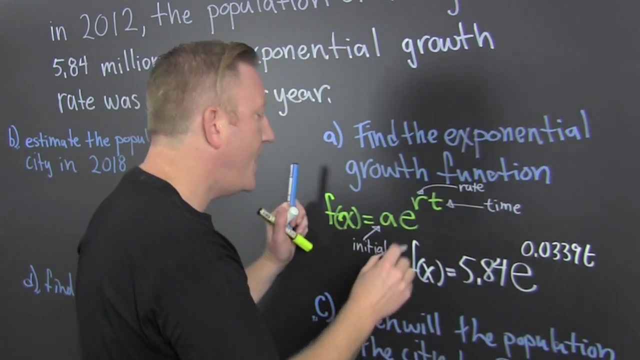 ooh, So then that's how we get 0.0, because I go, I go 1,, 2,, I fill it in, put a dot, All right. So then I write 3,, 3,, 9,, t. Can you see? Yeah, And there you go, That right there. 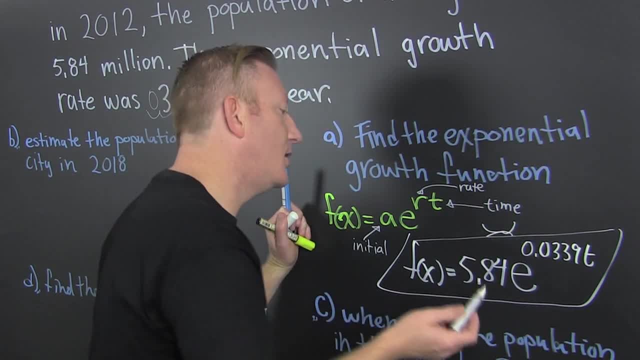 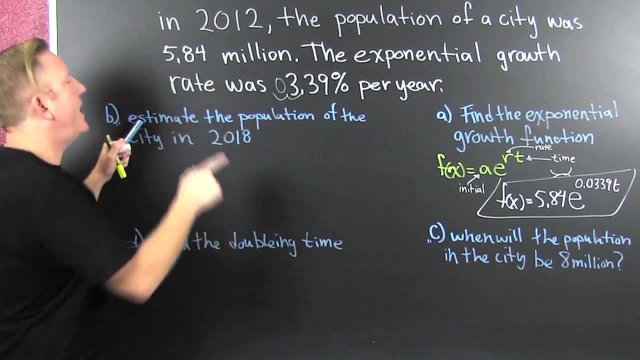 Pull it, Put it in a small purse. It's going to be clutched To the next question. What's the next question Over here in B? what are we trying to do? We're estimating the population of the city in. 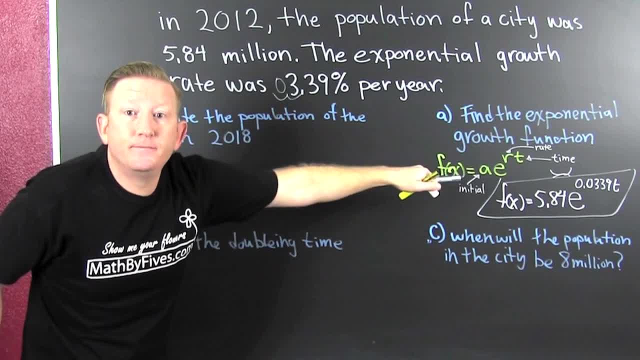 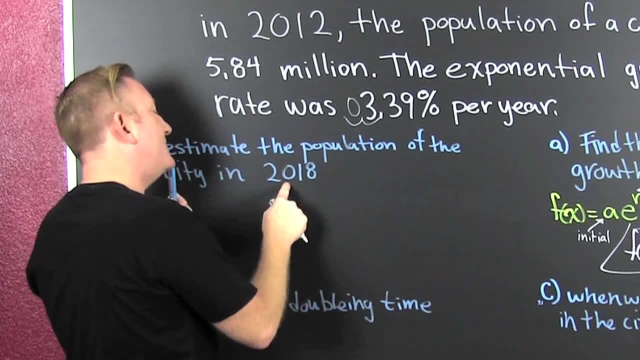 2018.. Now that t over there is times in years- What do we have? We're starting at 12, and we're trying to get to 18.. So you can do 2,, 0,, 1,, 8, minus 2,. 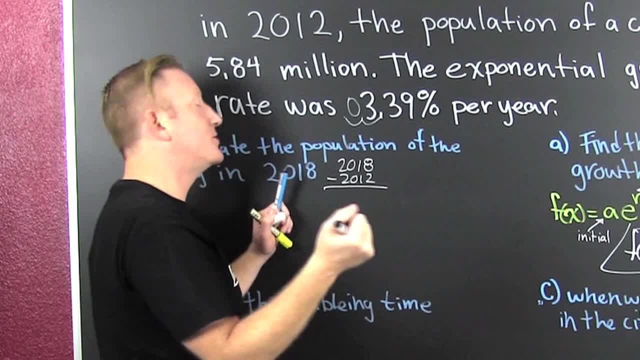 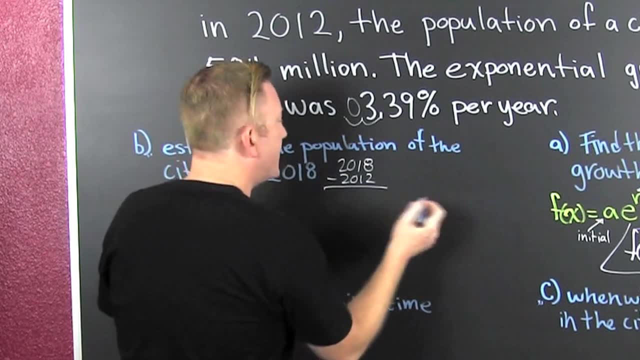 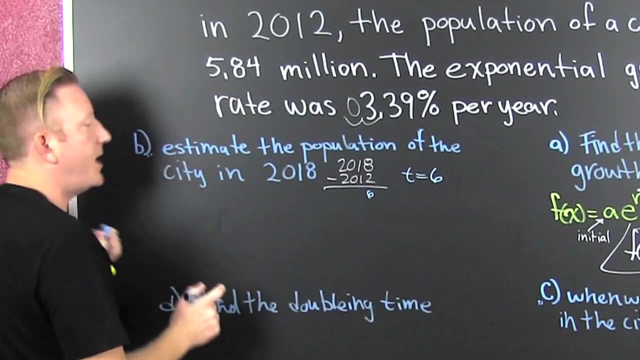 0,, 1,, 2, wait, You can count them down: 12,, 13,, 14,, 15,, 16,, 17,, 18.. So yeah, 6.. Here our t is going to be 6.. T is 6.. Then we plug it in there into our clutch. This is going to be f of 6.. f of 6,. 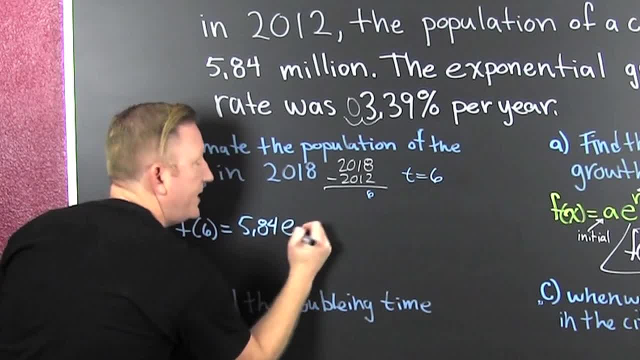 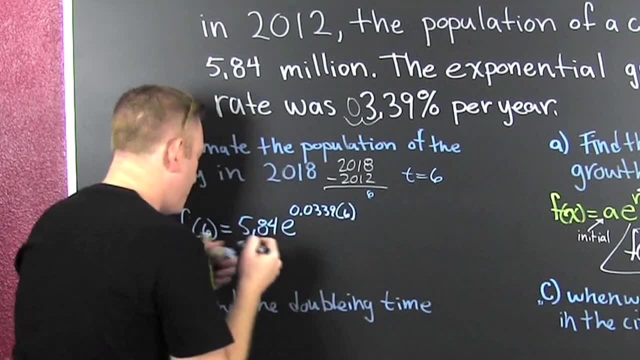 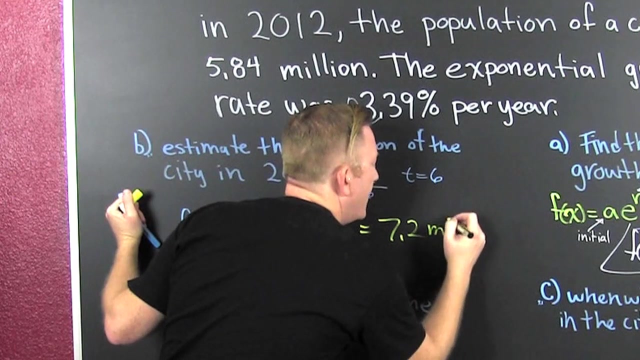 that's 5.84 e to the 0.0339.. Times 6.. And then when we pound all that out, boom, you put it in your whoa calculator, Sure. So upon computation you go and you get 7.2.. What's that? That's million, Yeah. 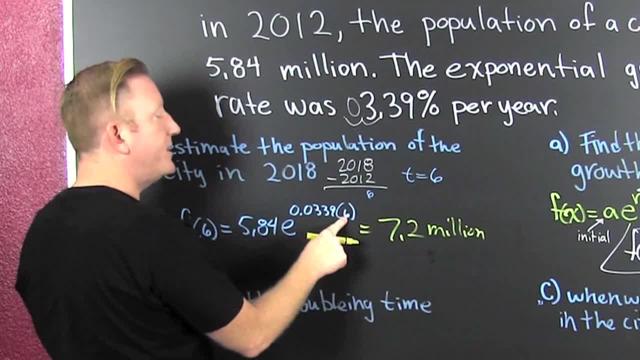 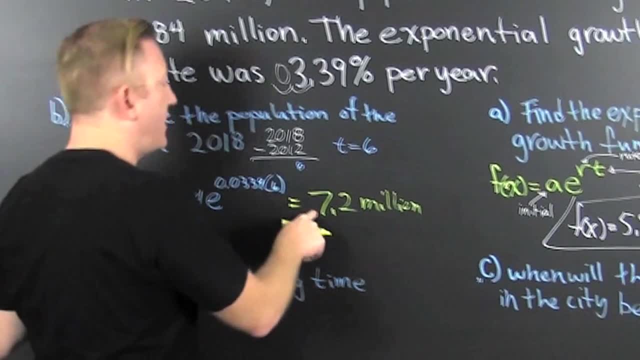 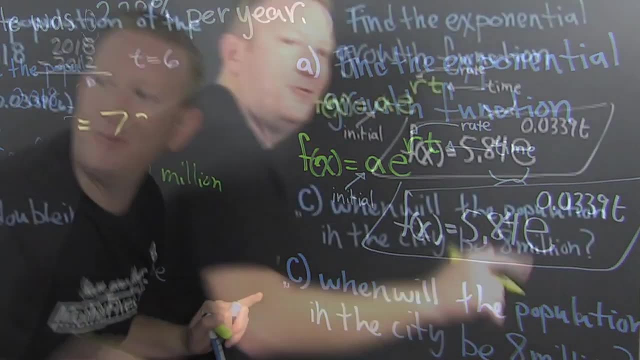 Why? Because what We put in time in years and we get out what We get out: population size in millions, So looks like 7.2 million. now Boom. When will the population be? You can't see that. We go over here. Come on, come on. 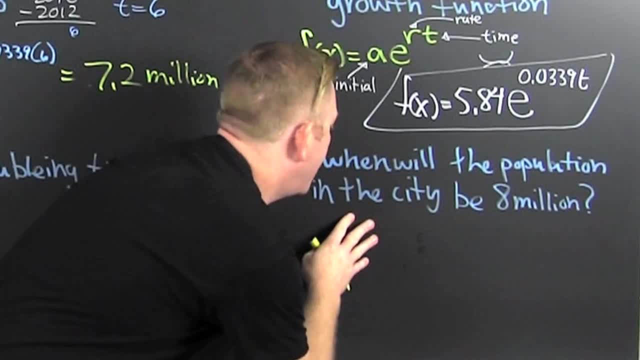 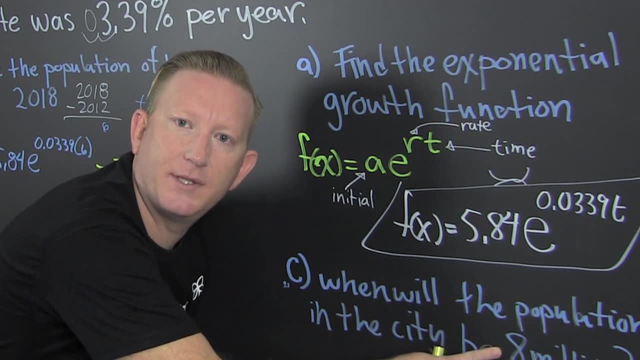 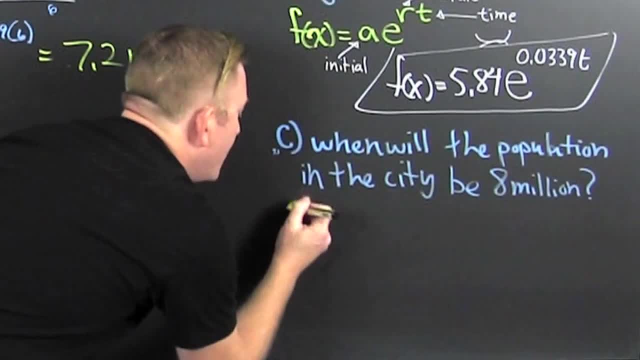 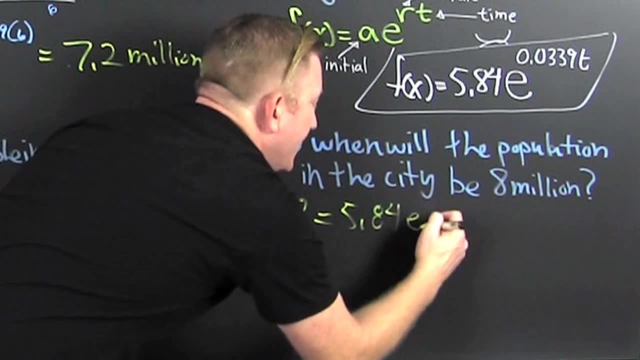 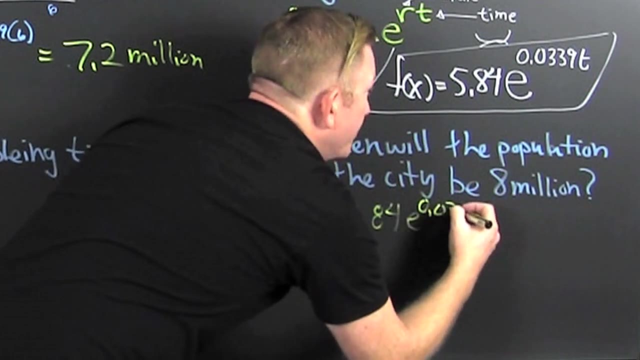 so we're going to put it on the out. Yeah, So on the outside we have 8 million. That's going to be equal to 5.84e to the 0.0339t. Now what do we? We divide by that? 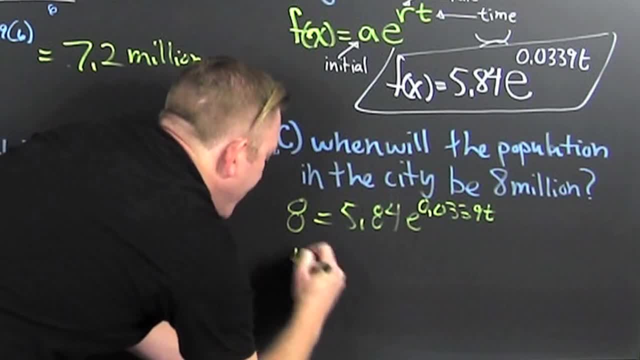 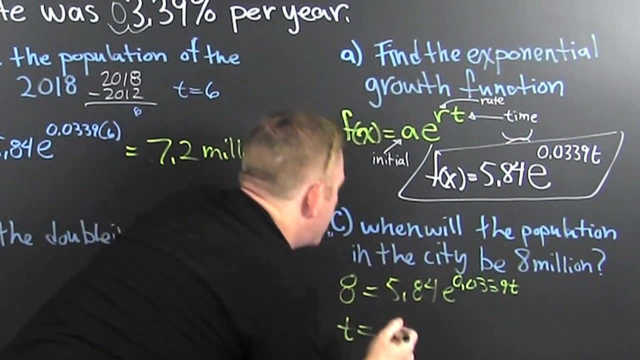 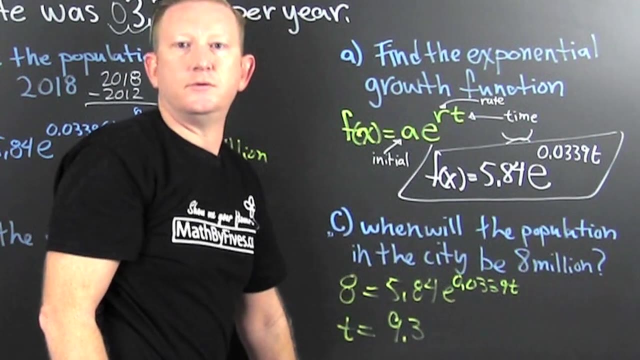 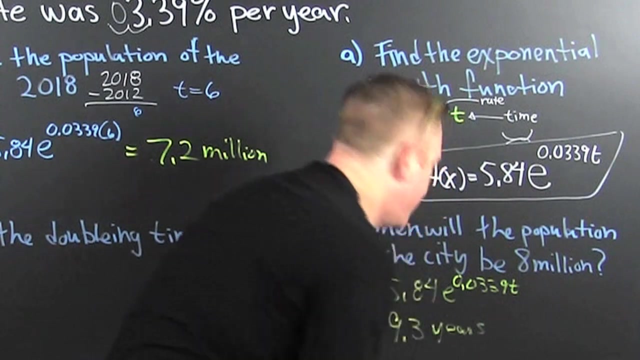 then we naturally log it. then we divide by that and we find that our t. I'll put the link of that in the description below. Maybe it appears here in some annotation. So t turns out to be 9.3.. What are the units on that Years? Yeah, Man, this is a brand new marker. 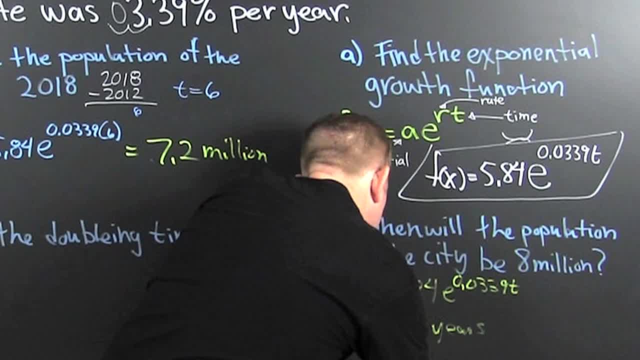 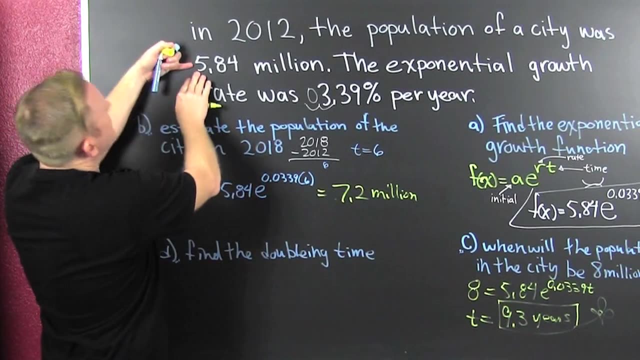 I don't know why it's acting up. That's a little better. A box of flour, Okay, come on now. Over here, Woo, We want to find the doubling time Dubbing. what do they mean We're talking about? it was at 5.84, and we want twice that. 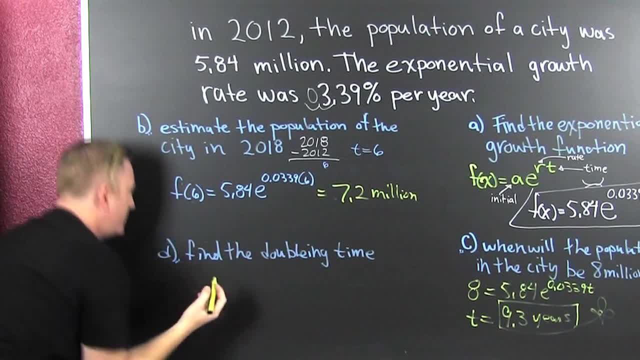 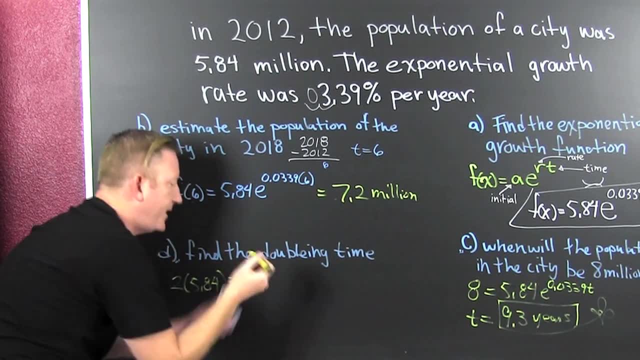 whatever it was, We can go and we can put. that we can do. we can do twice, that We can do 2 times 5.84.. That's going to be equal to. I can't even deal with this. Why does? 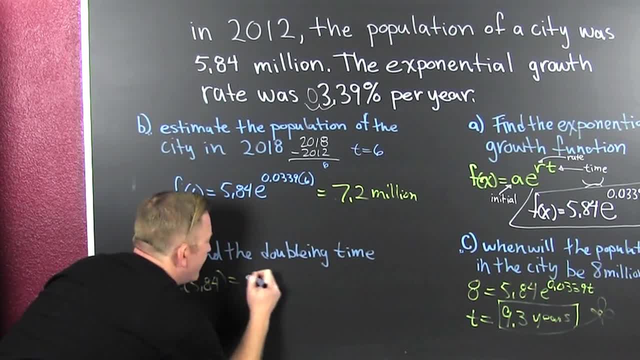 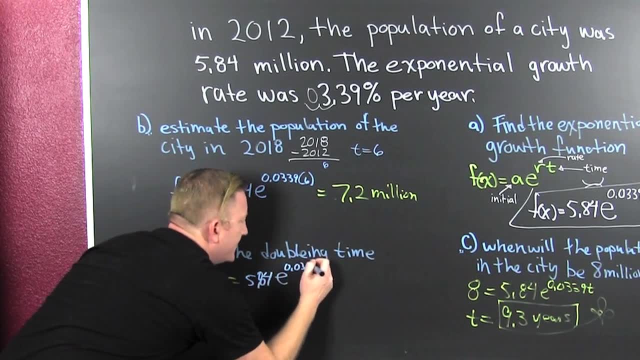 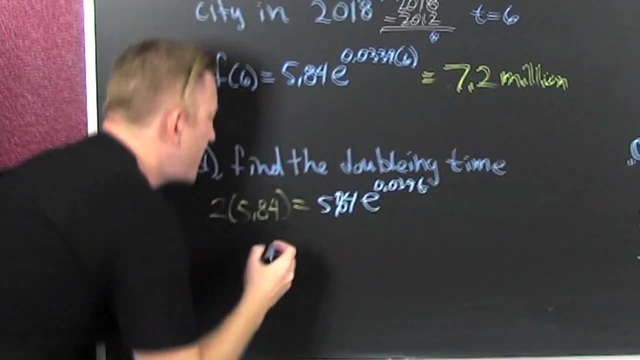 that even have a white top, 5.484e to the 0.039t. Whoa, We can do that, We can do twice that and then we can go and we can solve for t or we can do it in generally. what are we talking about? 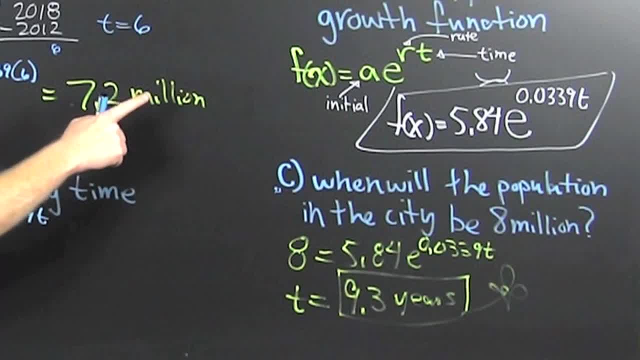 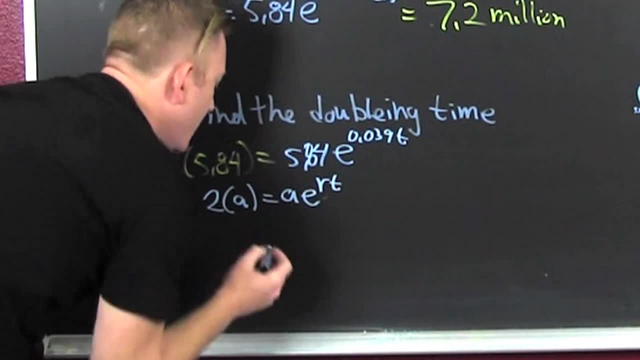 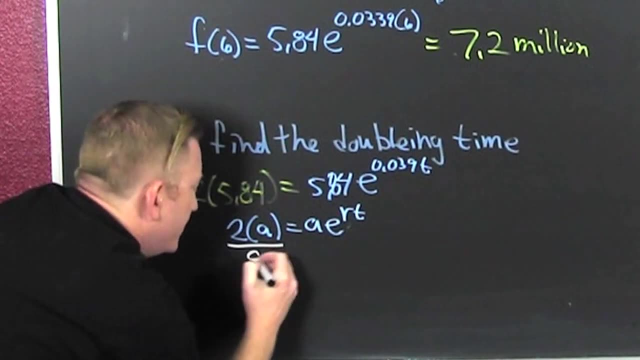 if we had two times a, what am i using? i'm using that general form over there. whatever a was e to the r, t uh-huh, but we knew our r, so, so so we divide both sides by. i need another marker. there's a white one. it doesn't have a top, so then, oh, a, a, okay.